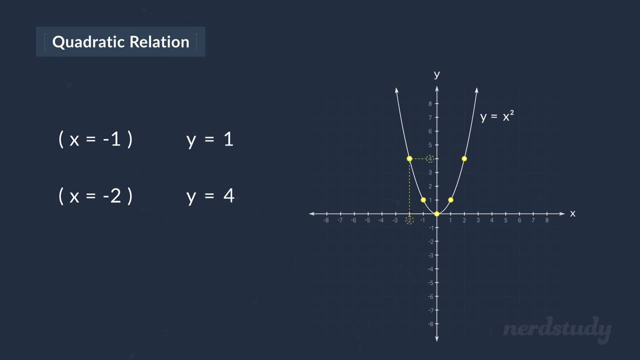 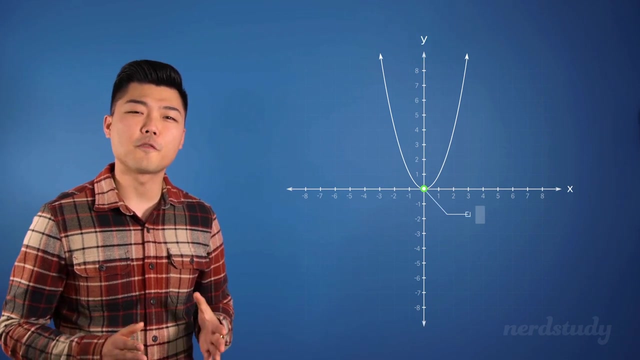 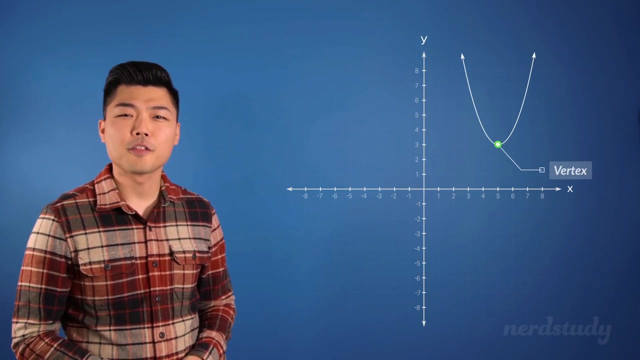 negative 2 multiplied by negative 2, giving us positive 4.. Notice how we plug in negative numbers and got the same value as plugging in the positive numbers. Great. Now this point right over here is called the vertex and, like we mentioned before, it does not necessarily have to be on the origin. The vertex can. 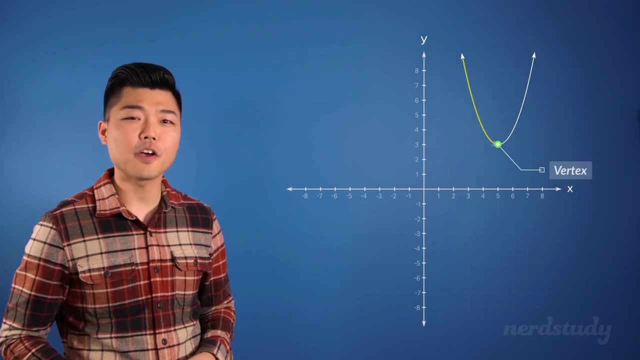 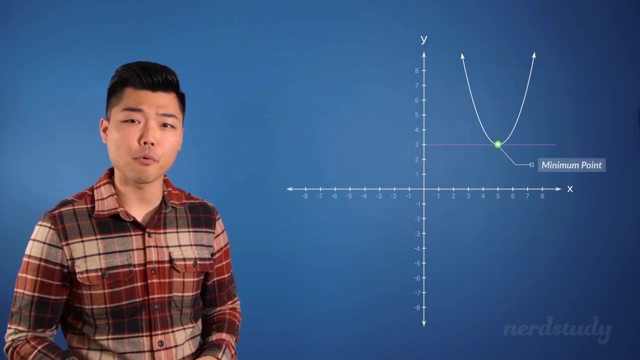 be thought of as the point in the parabola where the curve changes direction. If the parabola is opening up, then the vertex will be the minimum point, or shall I say the lowest point on the graph, If the parabola is. 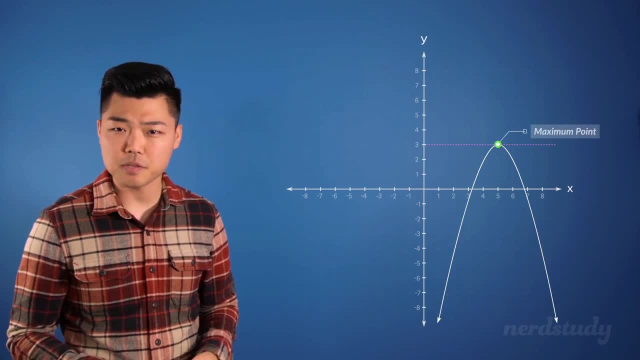 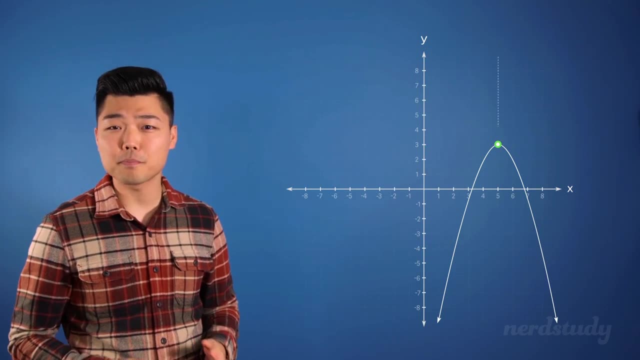 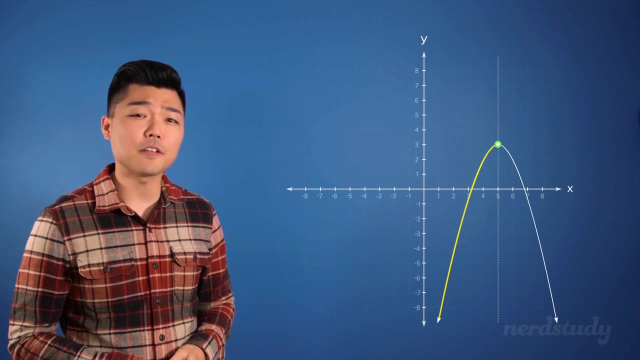 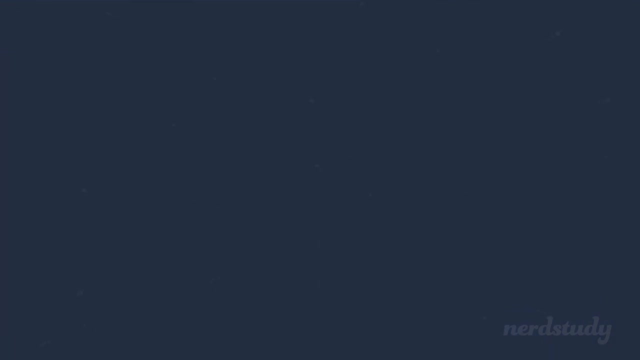 opening down the vertex will be the maximum point, which would be the highest point on the graph. Also, notice how the parabola is symmetrical to itself when it is seen as two halves. This imaginary vertical line that divides the symmetry of this parabola is called the axis of symmetry. So one way to tell if a 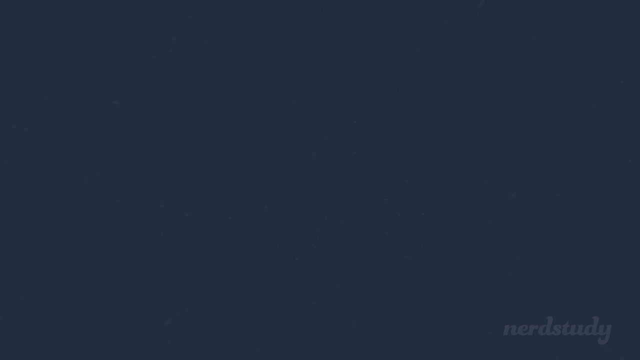 relation is a quadratic relation is by looking at the, the axis of symmetry. So one way to tell if a relation is a quadratic relation is by looking at the second differences of the y-values. Let's look at y equals x squared as our simple example to explore what second differences are. So the way we find them. 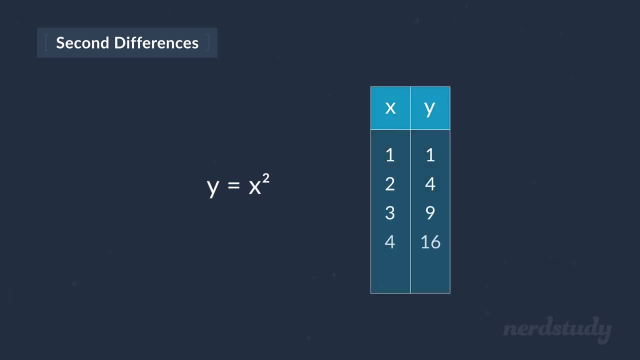 is by first creating a chart with the x and y values of this equation. Just make sure that the x values are evenly spaced out. In this example the x values are consecutive, so they go up by one. But if we wanted to, we could go. 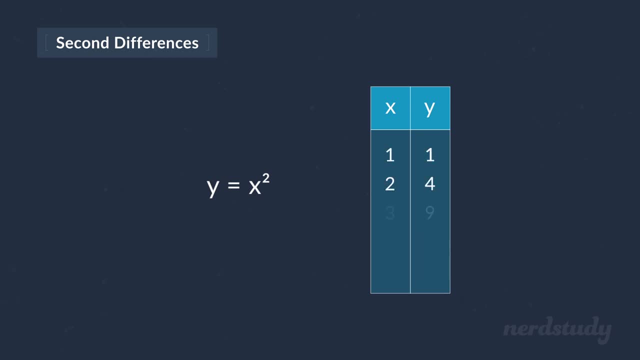 up by twos or threes or even any number, as long as they are consistent. So from here, let's add two more columns in our chart, which we will name as first difference and second difference. Now to fill the rest of the row of this first. 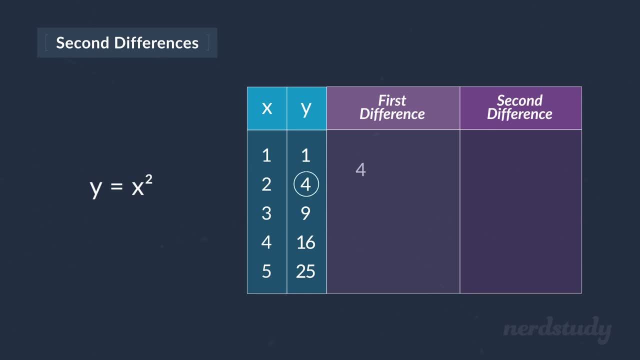 difference column. what we would do is get the second y-value and then subtract it by the first y-value. This gives us the difference between the two y-values. As you can see, we get three. Notice how we have it positioned in between the two. 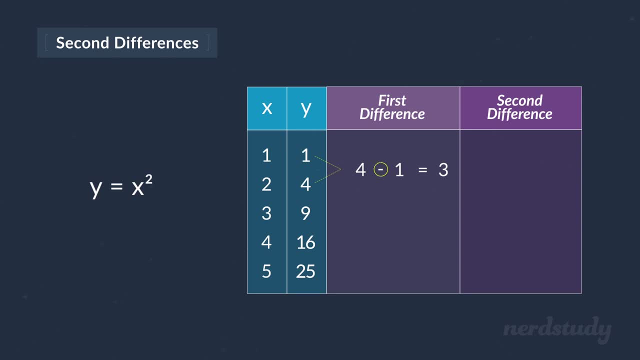 y-values to show that we are looking at the difference between these two particular values. Do this for several pairs of y-values. For example, the next one would be to get the third y-value and then subtract it by the second y-value. We write down our first difference again. 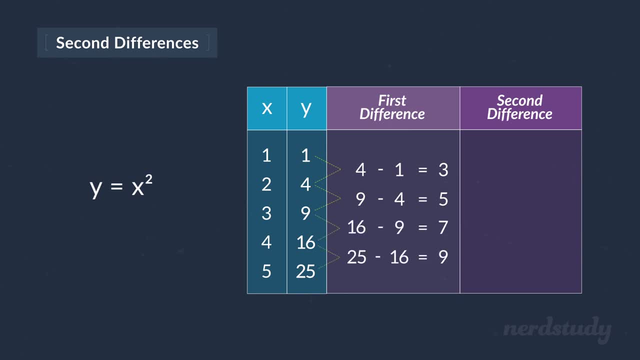 Try doing this again For two more pairs of y-values and compute the first differences. Now that we've got our first difference values, let's do the same thing that we did on this column, only this time let's do it over here. This is how we would get our 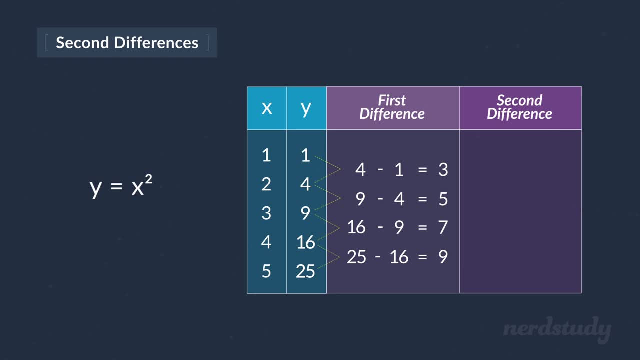 second differences. So again, we can just do second value minus first value, then we would do third value minus second value, Fourth value minus first value, Then we would do third value minus second value, Fourth value minus second value minus third value, and so on and so forth. 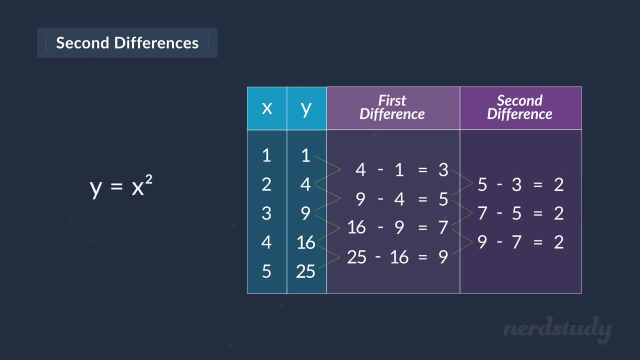 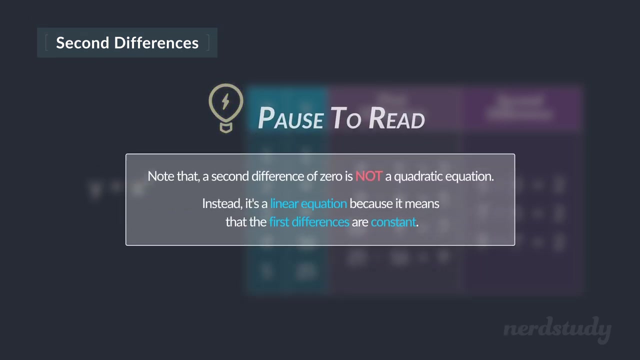 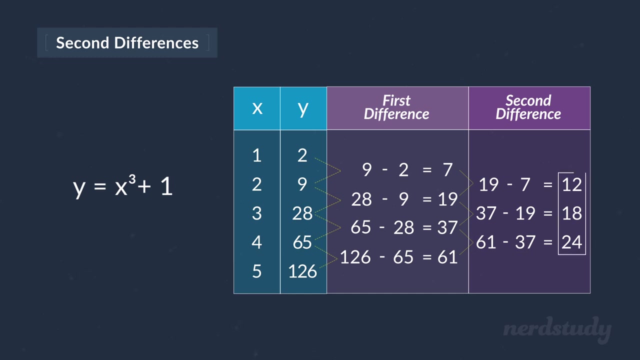 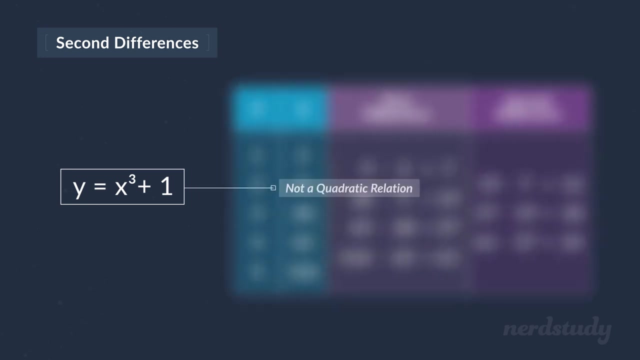 So what we should notice for quadratic relations is that the second difference will always be constant. This applies for all quadratic relations. So if you calculated the second differences properly and all the values are not the same or constant, then the equation is definitely not a quadratic relation. 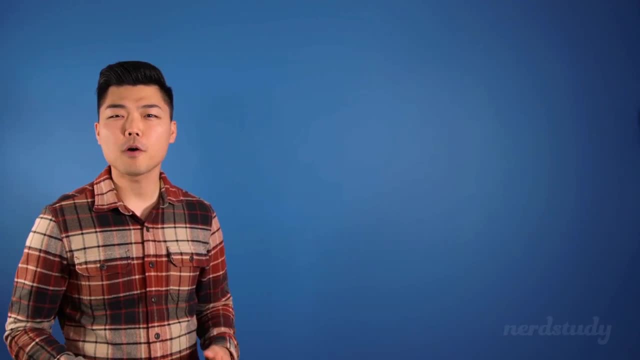 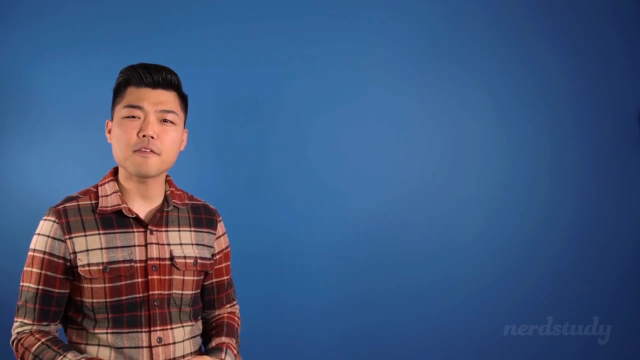 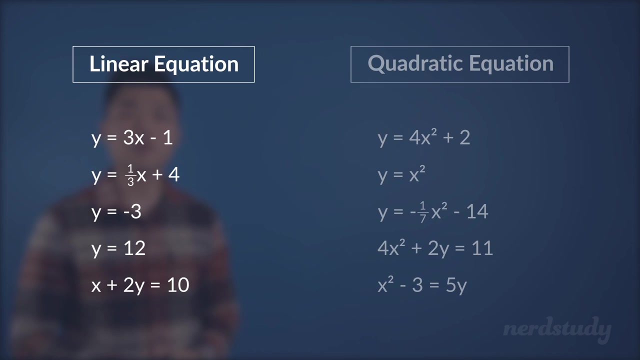 Awesome. So before we end this video, I want to compare what we know about linear equations with quadratic relations. A linear equation never has an exponent of 2 in it. Take a look at some of the linear equations on the screen. Notice how we don't have an exponent of 2 anywhere here. 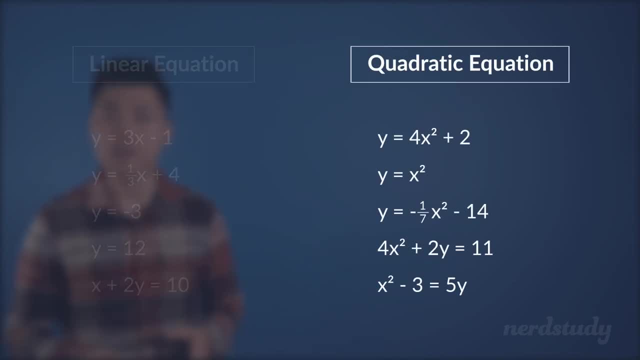 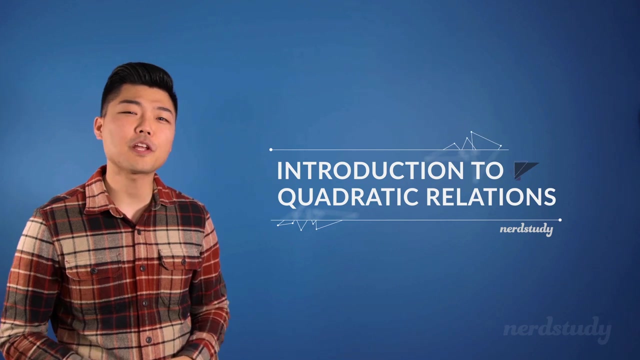 Now let's take a look at some of the examples of quadratic equations. For these, notice how there's an exponent of 2 on the x. This is something you can expect to see from quadratic equations. Well, that's it for this video on quadratic relations and the idea of first and second. 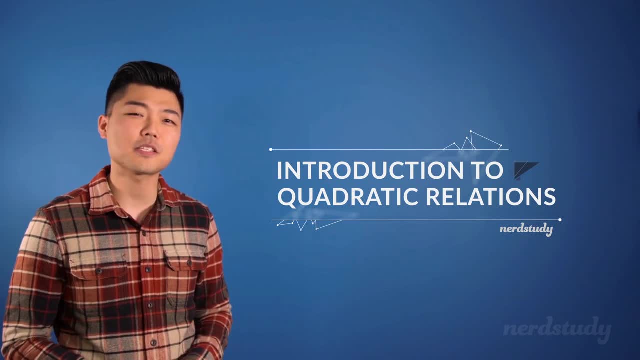 differences. Thanks for watching and we will see you in our next lesson.